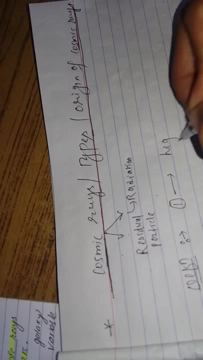 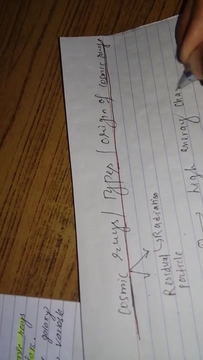 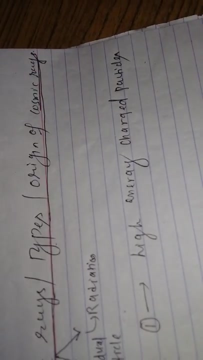 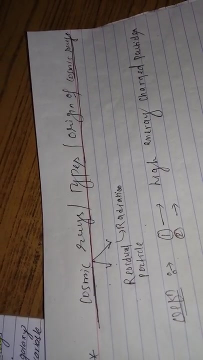 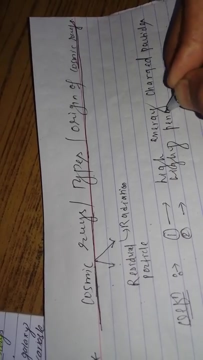 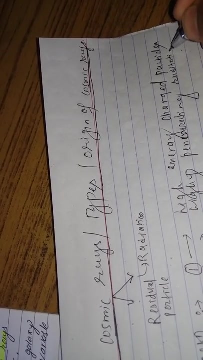 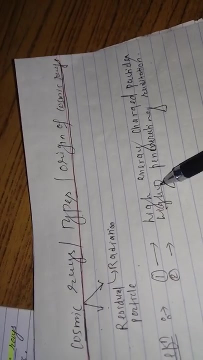 rays are those rays which are residual particles or radiations. What is residual high-energy charge particle? cosmic rays are high-energy charge particles. number two: cosmic rays are highly penetrating radiations. highly penetrating radiations in simply, the definition is: cosmic rays are highly penetrating radiations which are coming from the outer. 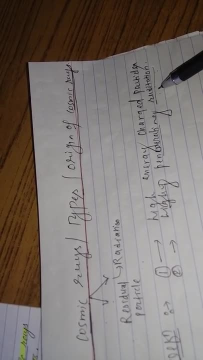 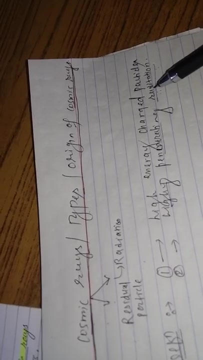 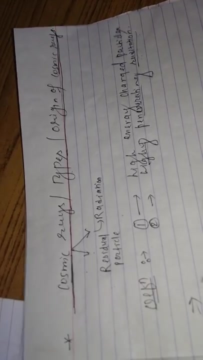 area of the solar system. so in this definition the cosmic rays are highly penetrating radiations, interstellar space and just strike into the bounties of our hot atmosphere in all direction. These cosmic rays are the very high energy charge particles. So its types number one is the primary cosmic rays. 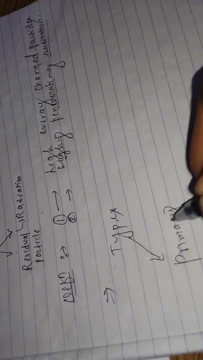 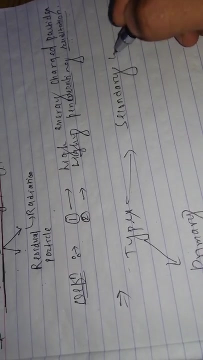 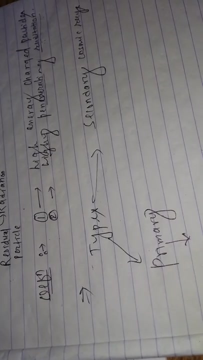 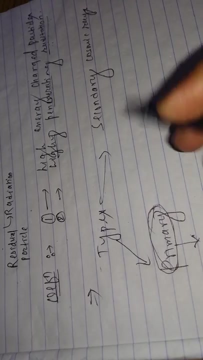 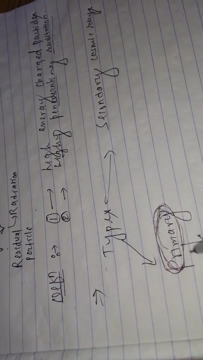 primary cosmic rays and next one is secondary cosmic rays. secondary cosmic rays: what are the primary cosmic rays? we know that the primary cosmic rays is simply the radiations just fall or strike on the hot atmosphere. these are the primary cosmic rays and one important point is that the primary cosmic ray consists of: 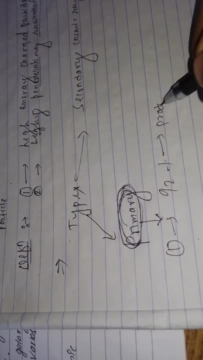 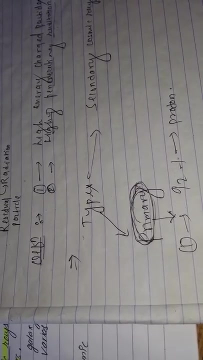 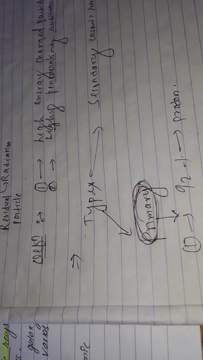 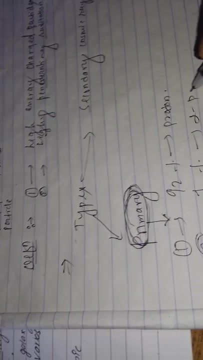 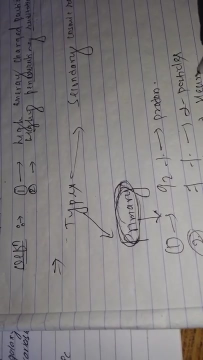 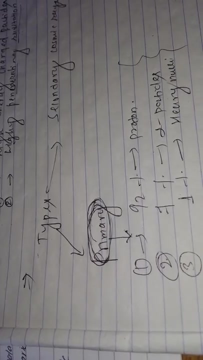 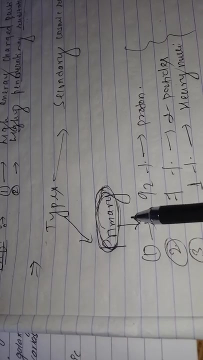 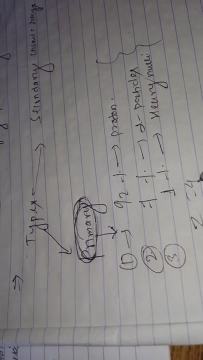 92 percent proton. 92 percent proton and number two is seven percent is alpha particle and number three is one percent is heavy nuclei. also remember that primary cosmic rays are the highly charged particles. the charge number z up to 40, all are the cosmic railings. that means primary cosmic rays. what is the secondary cosmic rays? secondary cosmic ray means the rays which are interact with the molecules in the outer stellar space. in i mean the molecules of continuous particles in the atmosphere of earth. and then they are they and these nature will be changes and nature will be changes and then fall into the boundaries. 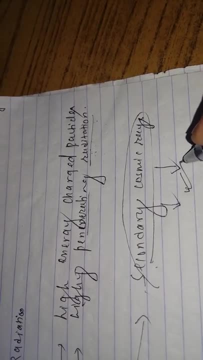 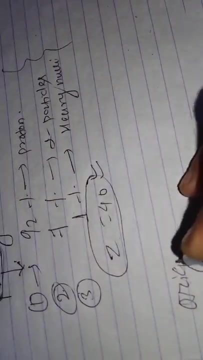 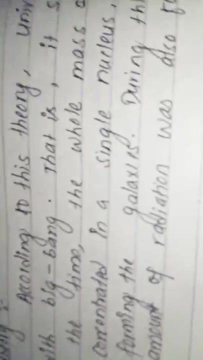 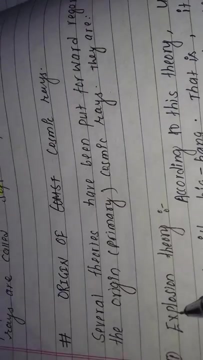 of earth atmosphere. these are called the second, the cosmic rates and origin of the cosmic rates and origin of the Toshimi grace. the cosmic raise the most. one important point is the explosion Theory. according to the explosion theory, the universe was started with the Big Bang. the 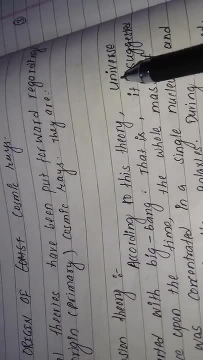 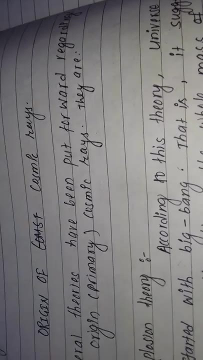 universe was he started with the Big Bang, that is, at that time. at the time of Big Bang, the whole mass of universe was constantly gone from one universe to another universe. at the time of Big, in a single nucleus. the whole mass of universe is concentrated in a single 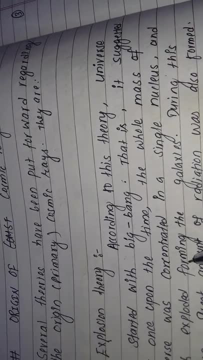 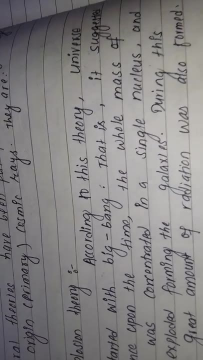 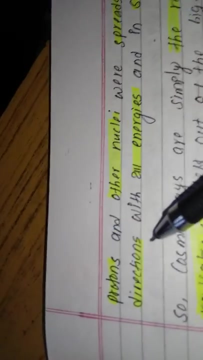 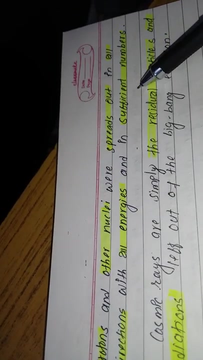 nucleus and which exploded, forming the galaxies. during this explosion, the grid amount of radiation was formed, so the proton and other nuclei. so the proton and other nuclei were. is spirits, proton and other nuclei. you spit it out in all direction with all energies and sufficient numbers. so simply the cosmic. 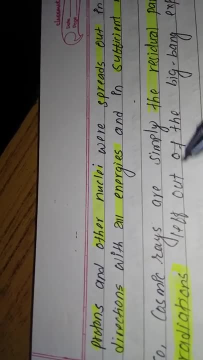 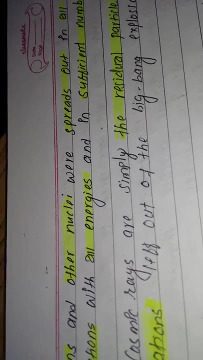 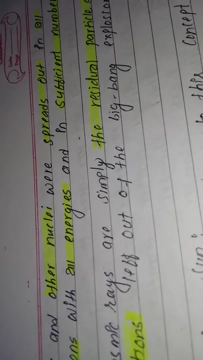 rays are the residual and the radiations left out from the big bang explosion. okay, according to the big bang explosion, we can say that the there's, that is the time. a big bang explosion, the whole mass of universe with my mask of universe in a who, if confined, nucleus may 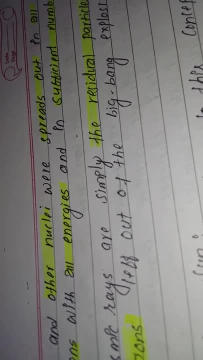 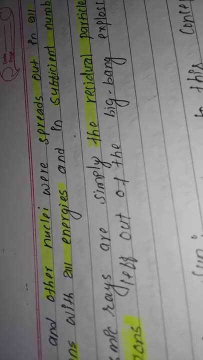 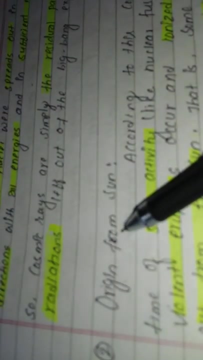 I mean the whole mass of the universe was concentrated in a single nucleus. At that time, a great amount of radiation was formed. Number two is the origin from the sun. Origin from the sun. What is the origin from the sun? What is the concept? 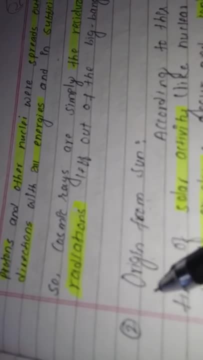 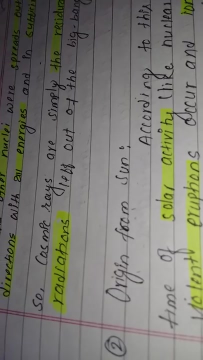 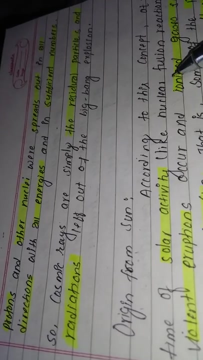 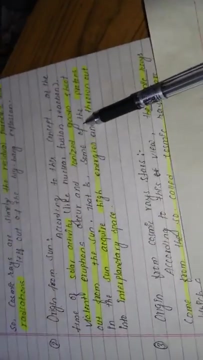 At that time of solar activity. at that time of solar activity, like nuclear fission or fusion reaction, like nuclear fission or fusion reaction, violent eruption and ionized gas shoot out from the sun. Violent eruption and ionized gas shoot out from the sun.